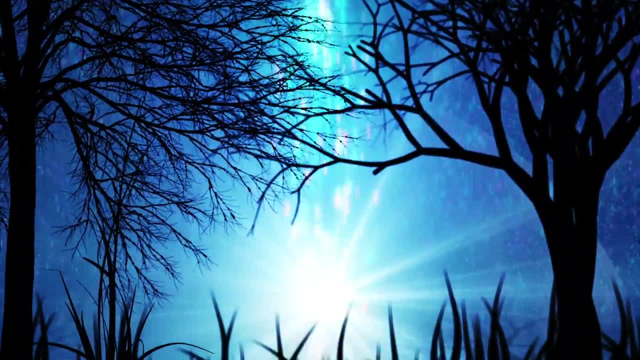 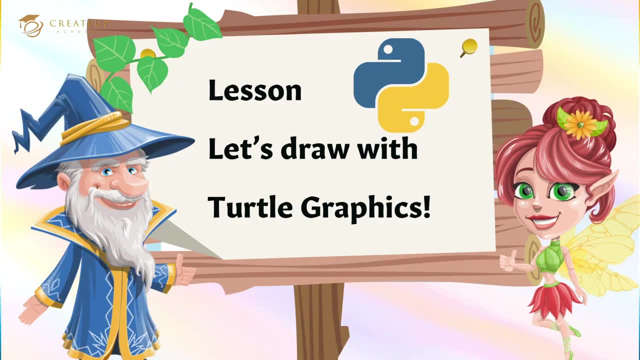 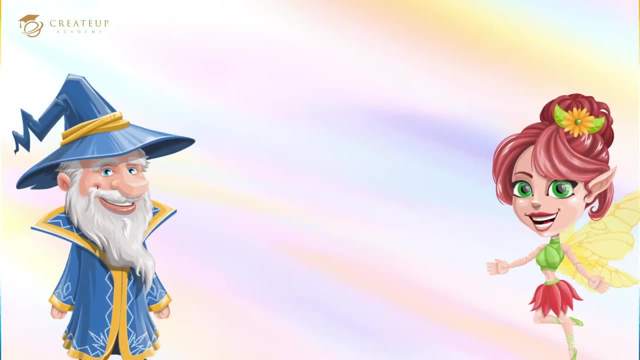 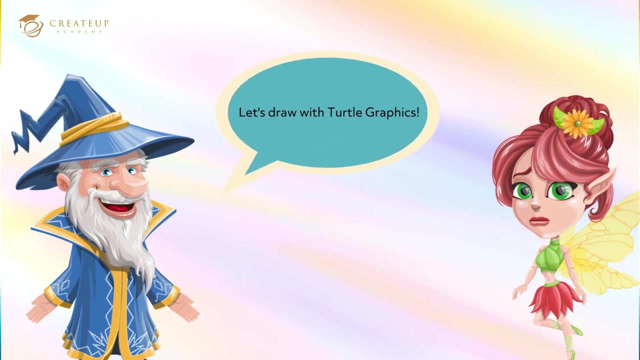 Let's draw with turtle graphics. Hey Liam, I'm getting a little bored just displaying the letters. Then let's try drawing. Let the turtle walk and draw a line. Sounds like fun, I'd love to try it. Let's draw a straight line with turtle graphics. 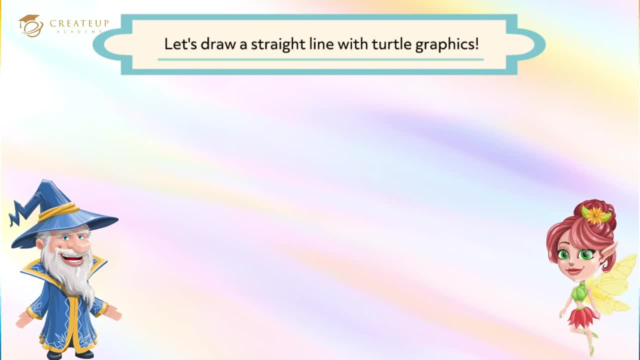 This program displays a straight line by moving the turtle straight ahead. First, let's open a new file from Idle and enter this program. What do these codes mean? This is an instruction to use turtle graphics. This is an instruction to make the turtle appear. 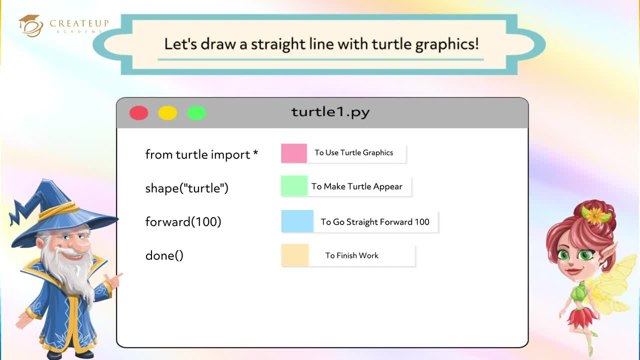 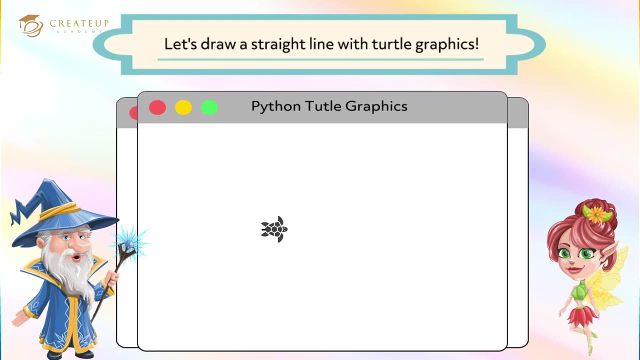 This is an instruction to go straight forward: 100.. This is an instruction to finish the work. I understand. Once you've written your program in a file, give the file a name and save it. Next let's run this program. When you run it, another window will open. 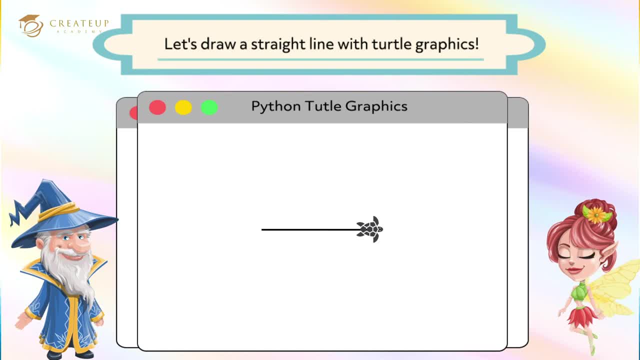 The turtle will walk and a straight line will be drawn. Oh, the turtle is drawing a line. Can this turtle walk back? You can make the turtle walk backwards with back, And you can also use left and right to turn the turtle sideways. 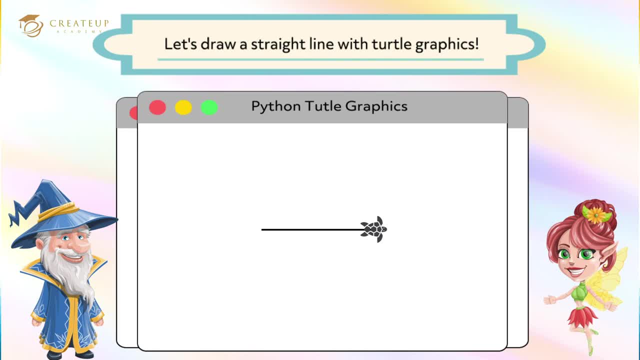 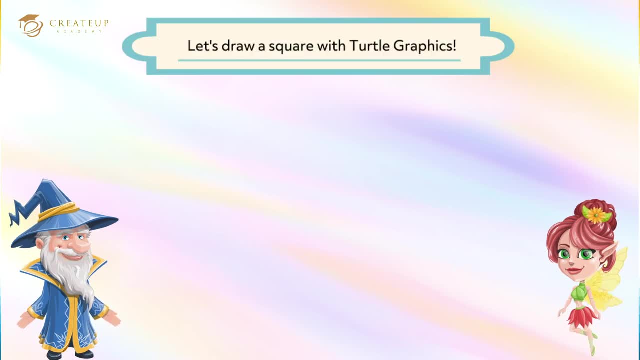 I found that I could draw a favorite picture by making the turtle walk in various directions. Let's draw a square with turtle graphics. Next, let's create a program to draw a square. Create a program to draw a square By repeating the go straight and turn 90 degrees. action four times. 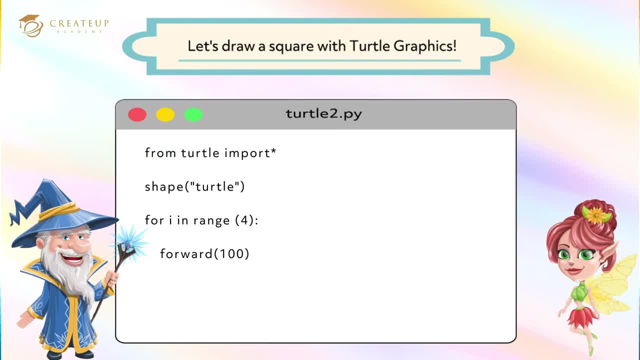 Now let's open a new file from idle and enter this program. What do these codes mean? This is an instruction to repeat the following process four times. This is a straightforward instruction to advance 100.. This is an instruction to turn 90 degrees to the left. 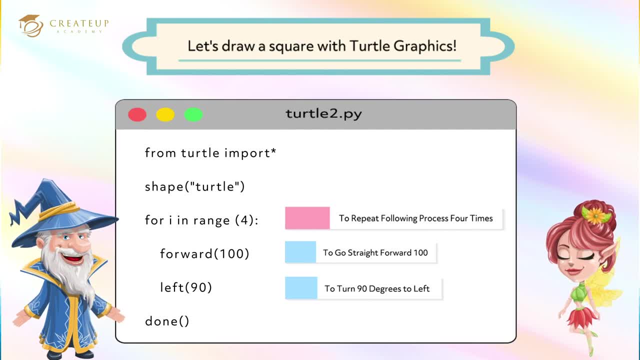 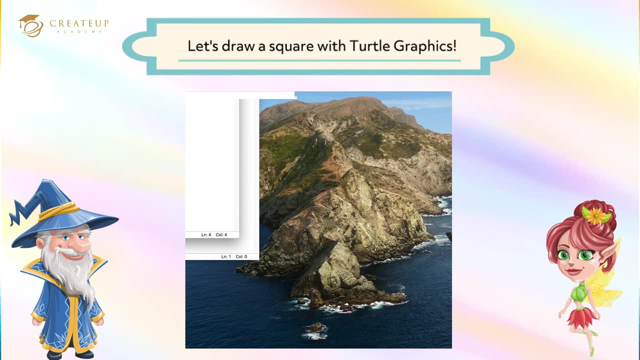 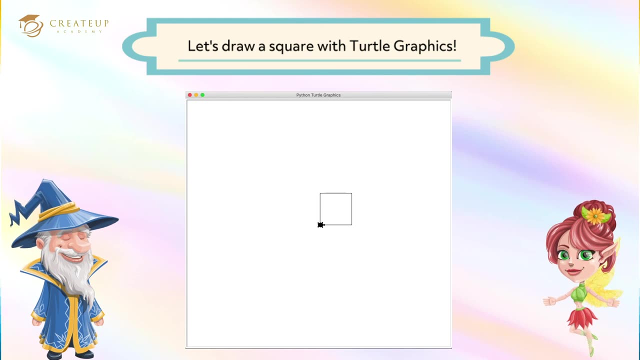 I understand, Once you've written your program, then a file. give the file a name and save it. Next let's run this program. Wow, the turtle drew a square. By the way, are the four squares at the beginning of the line necessary? 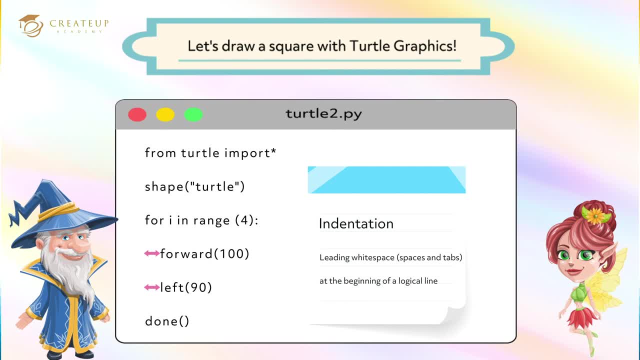 It's called indentation and it's a necessity. What is indentation? Indentation is entered with the tab key or space key. indentation is entered with the tab key or space key. indentation is entered with the tab key or space key. However, idle has an automatic indentation feature. 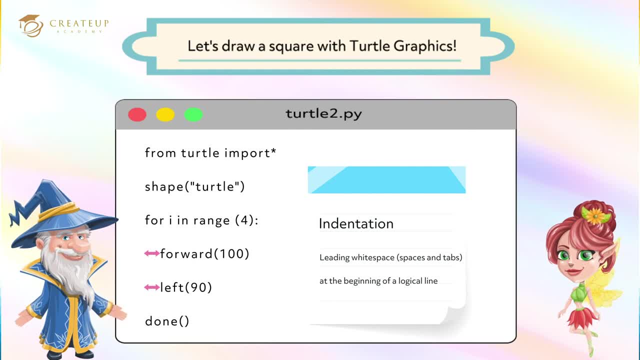 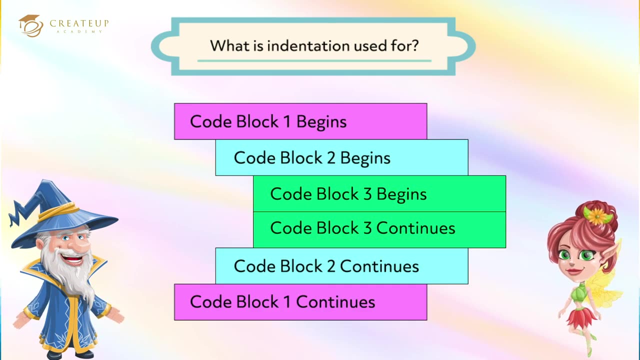 If you don't need the indentation, you must remove it yourself, Since indentation makes sense in Python. putting indents where you don't need them will result in an error. What is indentation used for Python? indentation is a way of telling a Python interpreter. 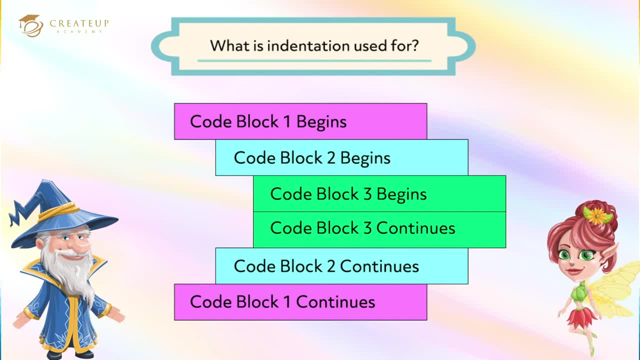 that the group of statements belongs to a particular block of code. A block is a combination of all these statements. Block can be regarded as the grouping of statements for a specific purpose. Python uses indentation to highlight the blocks of code. All statements with the same distance to the right belong to the same block of code. 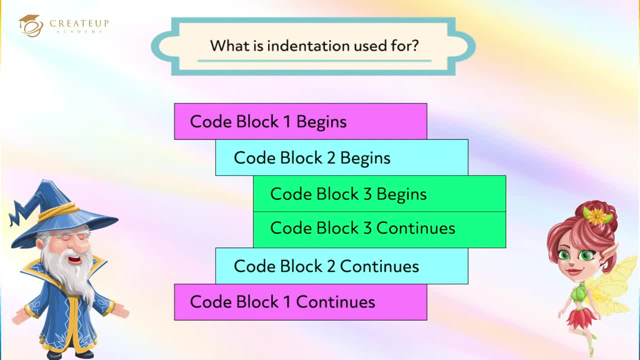 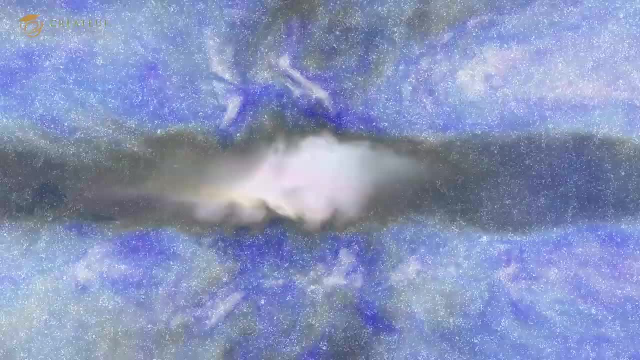 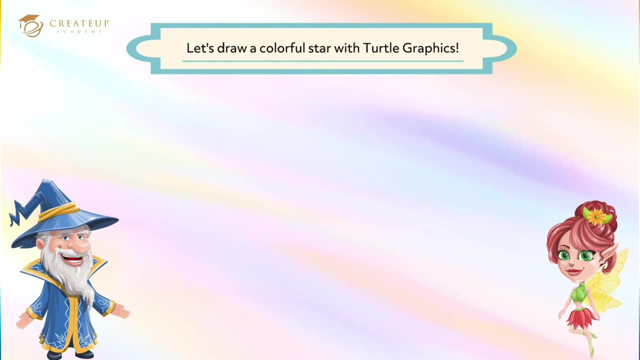 If a block has to be more deeply nested, it is simply indented further to the right. I now understand the indentation. Let's draw a colourful star with Turtle Graphics. Next we will create a program to draw a colourful star. You can draw a star by repeating the action. 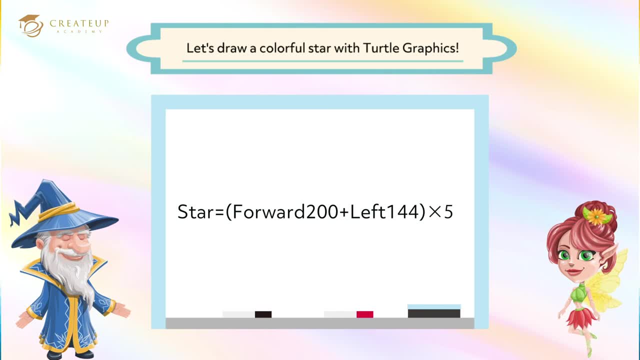 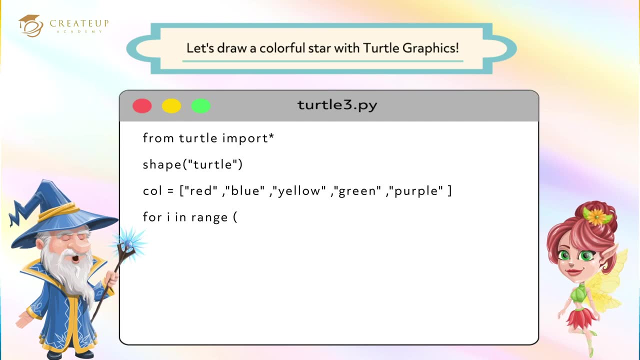 go straight and turn 144 degrees five times. This time we are going to colour in the lines, So let's open a new file from idle and enter this program. What do these codes mean? This is an instruction of the colours to use. 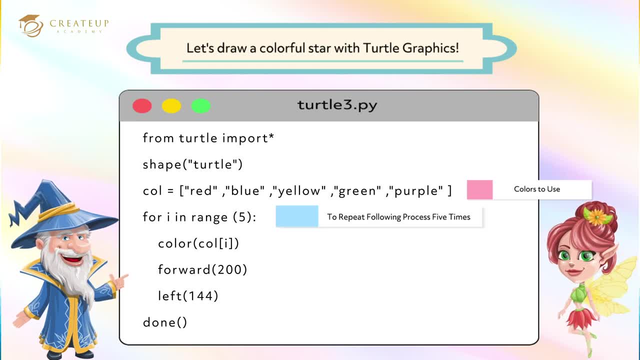 This is an instruction to repeat the following process five times. This is an instruction to change the colour of the line. This is an instruction to advance 200 straight ahead. This is an instruction to turn 144 degrees to the left. Once you've written your program in a file, give the file a name and save it.